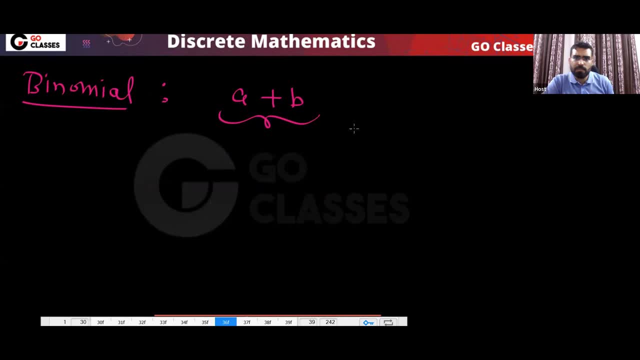 thing is called binomial. Ok, a plus b, Where a, comma, b are real numbers. They can be any real number, So this thing is called a plus b. This is called binomial. Binomial means summation of two numbers, Summation of two numbers. That is your binomial. Now you already. 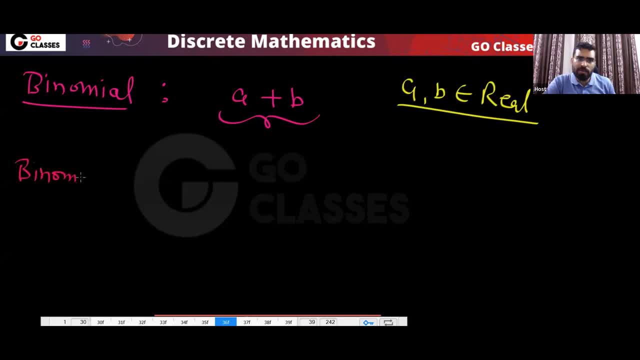 know? And what is binomial theorem? What do we mean by binomial theorem? Binomial theorem says that if you have two values, a plus b, then what is their power? n, Where n is a natural number. n must be a natural number. 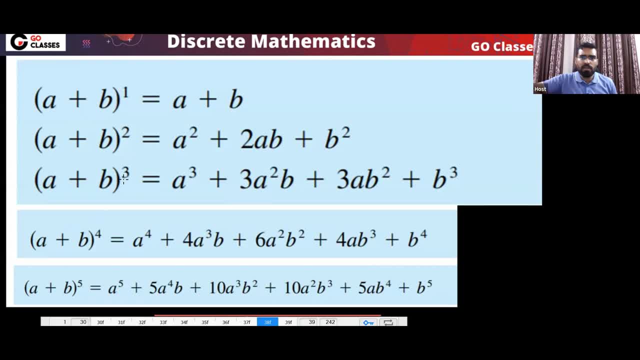 So, for example, What is their power 1?? What will be the power 1?? That will be a plus b. What is power 2?? This is your favorite formula from school life: a square plus 2ab plus b square. What? 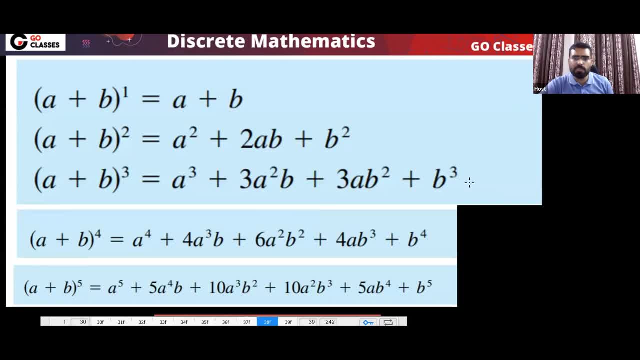 is power 3?? That is a cube plus 3a square b plus 3ab square plus b cube. Only these, we remember These. we don't have to remember, Only these we remember. We need to remember these now. Ok, So let's move on. How we can get a plus b power 10?, For example, Let's. 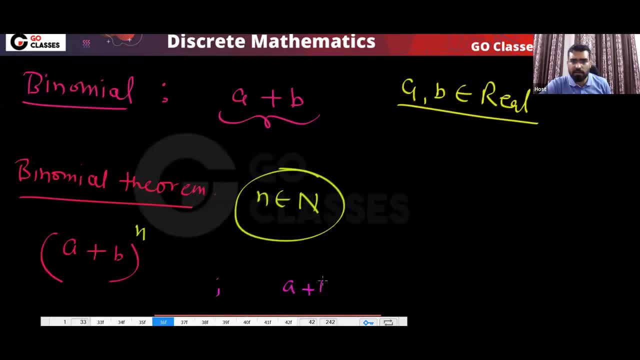 see how we can get a plus b power 10.. How will we get this? So this idea? So let's understand each of them one by one. If you do a plus b square, a plus b square, What does this mean? That means a plus b multiplied by a plus b. Correct, This means a plus b multiplied. 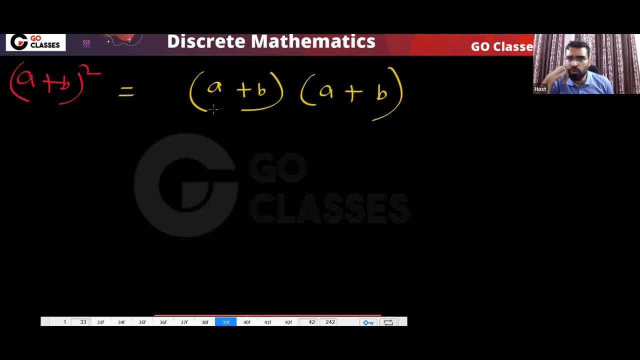 by a plus b. Now what you can do: See total, two terms you have here In this product. you've first and you have second, So let me call it one and let me call it two. Okay, so you have two things, one, two. Now how to multiply from this one you can take a yes or no from. 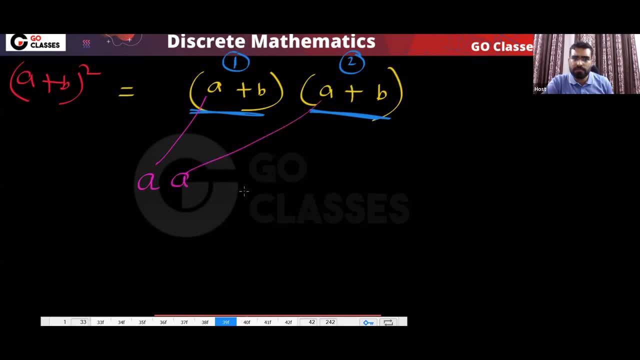 this one. you can take a from this two. you can take a or or or what I can do from this one. I can take a from this two. I can take b or what I can do from this one. I can take b from this two. you can take a or what I can do from this one. you take b and from this. 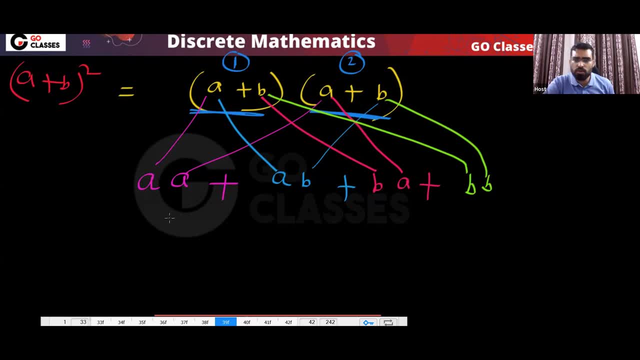 two, you take b. So this you will get. okay, yes or no? So finally, can you notice this and this: they are same: a, b plus b, a, these are same. So finally I can say: a power two plus two, a b plus b square. This is your formula, But few interesting things you should understand. 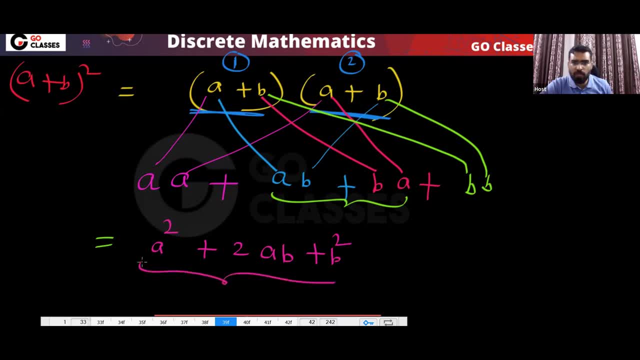 You should understand. You should understand few interesting things. What, finally, how many terms do we have? Finally, how many terms we have? We have total three terms. Finally, we have total three terms. Can you notice, in all the terms, number of a plus number of b, that is two right number. 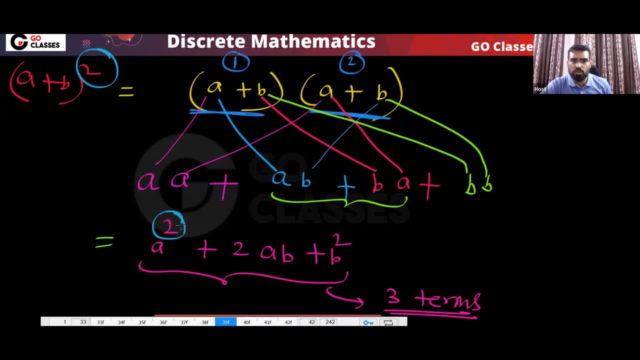 of a plus number of b, that is two. Like here, number of a is two. Here number of a plus number of b, that is two. Here number of a plus number of b, that is two. So number of a plus number of b, that is always two. 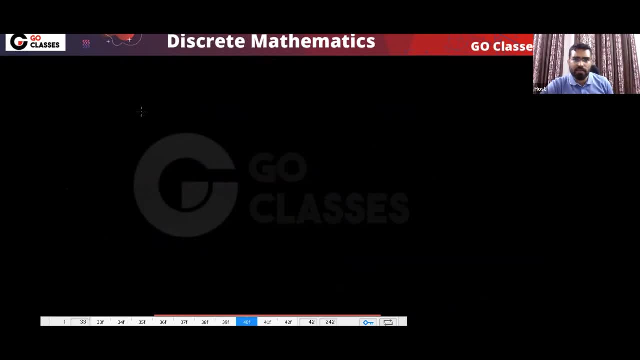 Why this is happening. This is happening because of this: You have a plus b. you have a plus b. Now let's think about in some different way, some different way. We will think you know one thing, one thing: you can get into that: whatever term, I will get Whatever term. 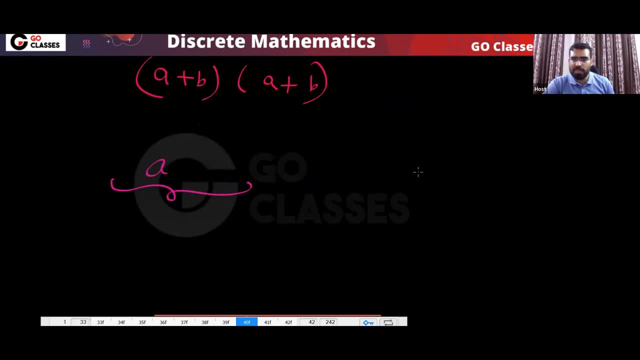 I will get number of a. there will be some a. there will be some b's, yes or no? There will be some a's, there will be some a's and there will be some b's. How many b's will be there? If number of a is k, then how many b's will be there? Two minus k, Right, Yes. 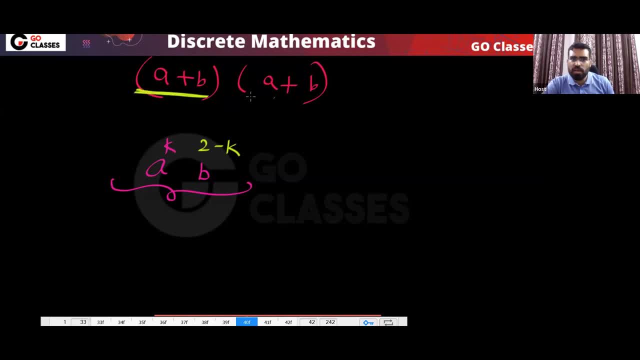 or no, Because if you are getting okay, there are total two terms. So if you are getting k a's, then you will get two minus k b's. Now, how many ways you can create this term, This term, in how many ways you can create This term in how many ways, For example: 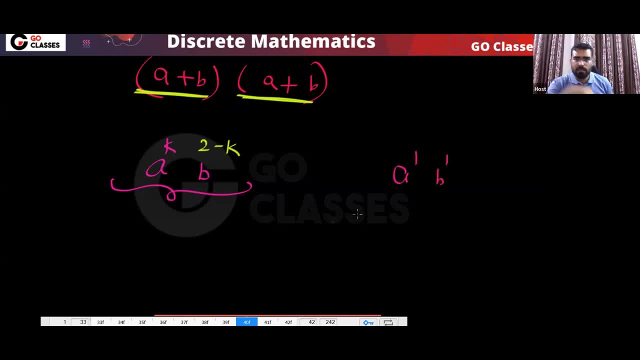 this term, this term. how many ways you can create, To create this term, you need one, a. Okay, just understand. please understand this: How many ways we can create this term? This is my question: How many ways you can, how many ways we can create this term? We? 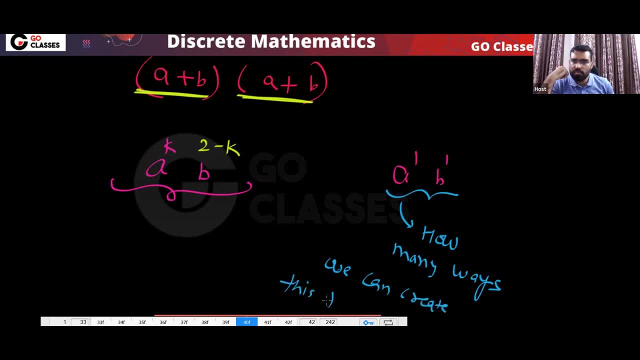 can create this term. So, to create this term, if you want to create this term, then from either from this or from this, we need one, a. So from these two, we need one: a. Either from here, you need a, or from here you need a. So, from these two, from one of them, you 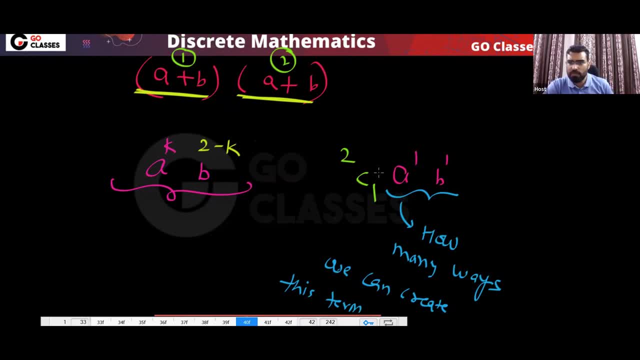 need a From the remaining automatically. b will come From the remaining automatically, b will come. So this term, in how many ways you can create So this term? in how many ways you can create Two ways? This term you can create in two ways. Okay, because this. 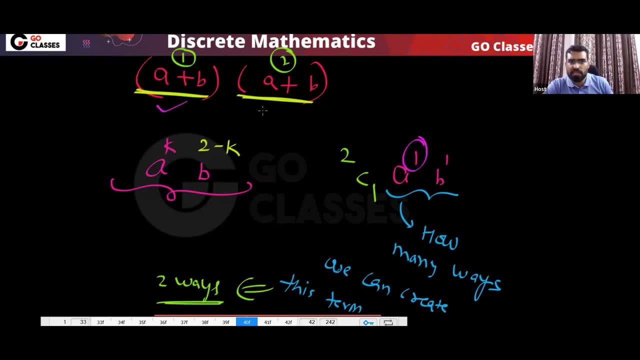 term, you need one, a. So there are two things: Either from here you take a or from here you take a. So there are two things From them. from one of them you will take a. From the remaining, who will come From the remaining? like from here. if I take a, then from here. 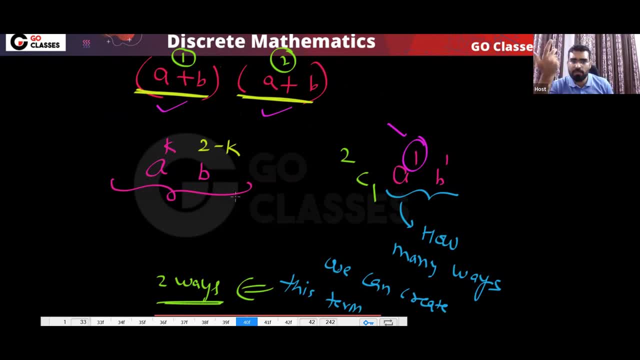 who will come b From here? b will come. Okay, So now tell me how many ways you can create this term, This term. in how many ways you create? You need two a's, So from both of them you should take a, So this term you can create. 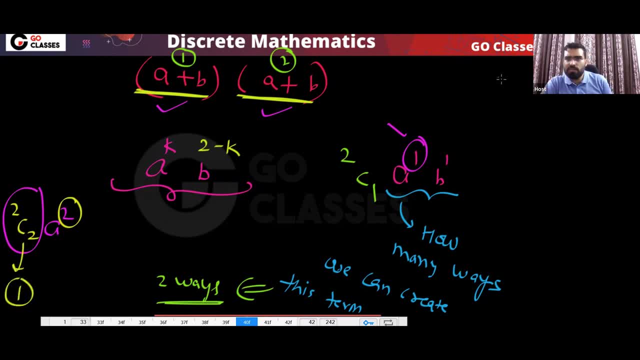 in only one way And in how many ways we can create this term, This b square, In how many ways we can create. So, from these two, from this and this, from these two, you select two And from both of them you should take b From here. b should come from here, b should. 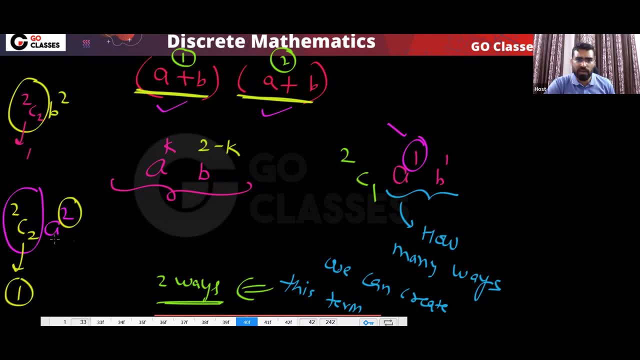 come. So this term also, I can create in only one way. So this is your answer. So, finally, you can create in one way, So this term you can create in one way. From both of them you take a. So I can say: this term you can create in one way, Plus this term you can. 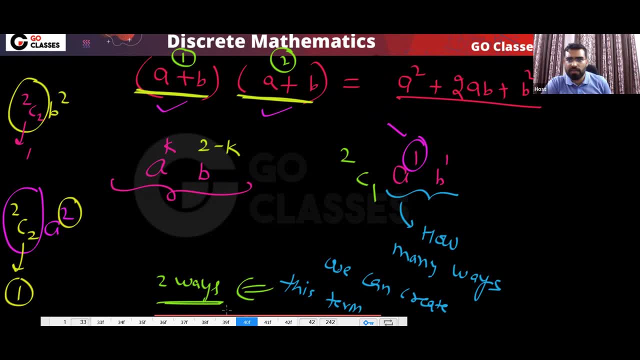 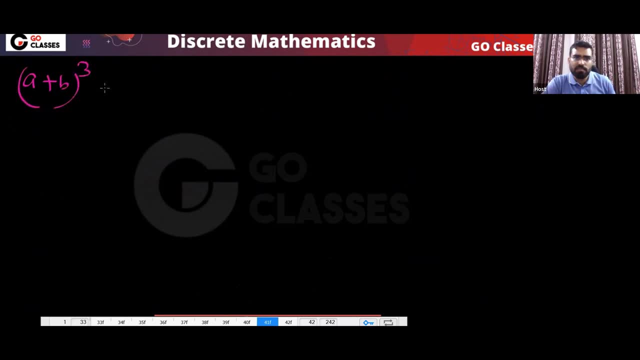 create in two ways. Plus this term, you can create in one way. Let's see this one Now. let's see a plus b power. a plus b power- 3. What that will be, a plus b, a plus b a plus. 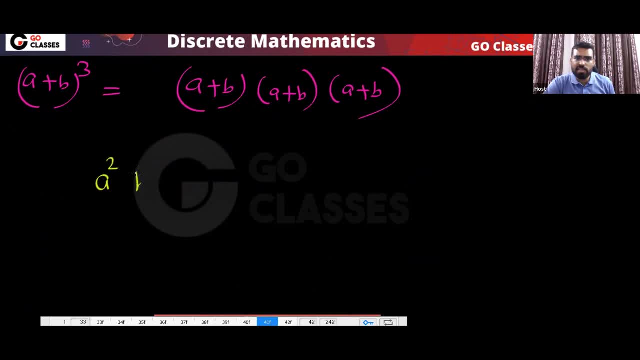 b. Okay, How many ways I can create this term. I want to create this term, How many ways I can create this term To create this term. you have total three things. You have one, two, three, So basically decide from where you are taking b. See one b you want, How many b you want. 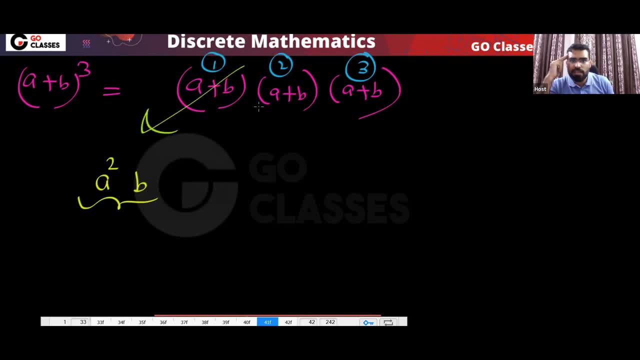 You want one b, So either you can take b from here, Then from here who will come, Then from here who will come a From these two a will come. So what you can do, Either from here you can take b, or from here you can take b, or from here you can take b. 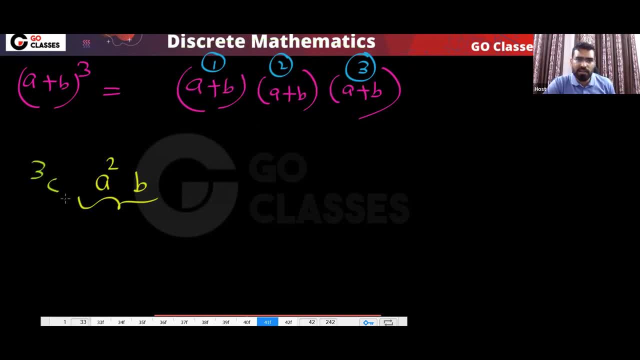 So there are total three things. From these three things, you can decide who will give you b. You can decide who will give you b. So this term will come with this, And how many ways you can create this term. How many ways you can create this term, This term, how. 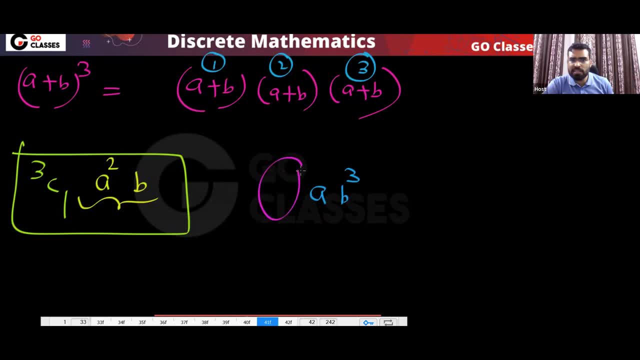 many ways you can create Zero way You cannot create this term. So this term you cannot create, This term will be created in zero ways. This term will be created in zero ways. How many ways you can create this term? So, from all of them, all of them, a should come From all. 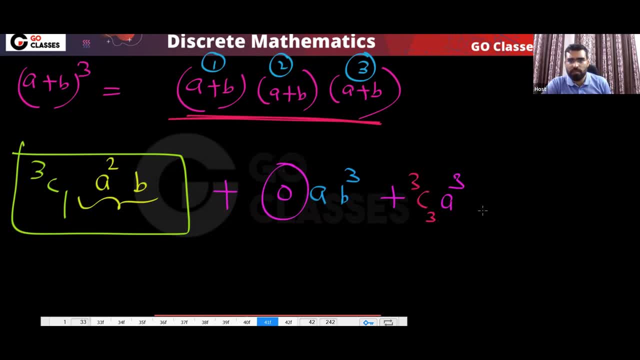 of them, a should come. So from all of them, a should come From all of them. a should come Only one way. So this term you can create in only one way. How many ways you can create this term? a, b, square, This term, again, you can create in three ways, Like from zero to. 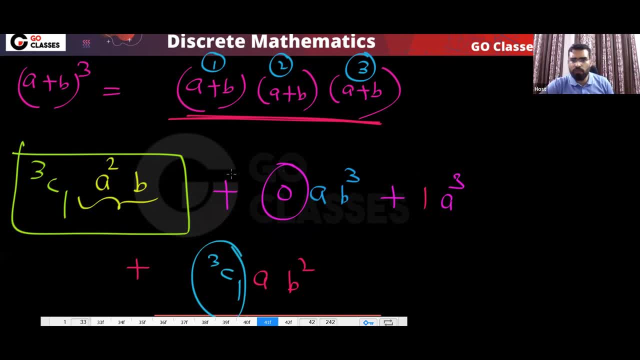 zero. You can decide who will give you a, Who will give you a. you can decide Like: this will give you a, or this will give you a, or this will give you a. So this you can decide. So this is the idea. Now, that's it. This is the final answer. This is your final step. 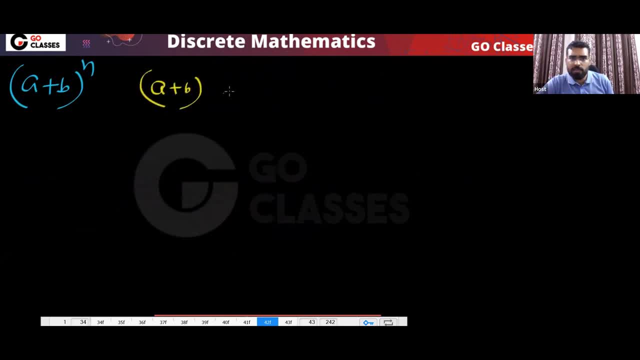 If you have a plus b, power n, then you have a plus b, a plus b, a plus b, and so on, a plus b. So total, how many a plus b, you have Total n. One, two, three, four, five, six. 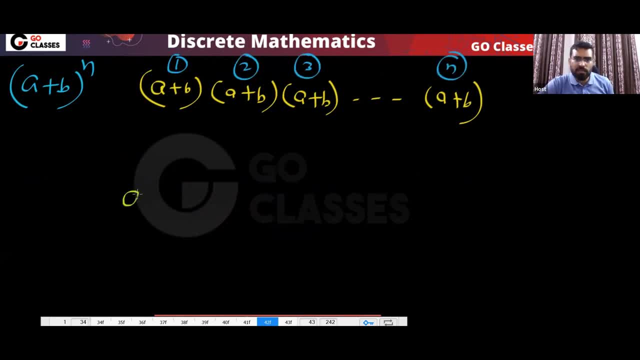 seven, eight, nine, 10,, 11,, 12, 13 total n a plus b. you have This term. how many ways you can create a power r b, power n minus r? See if you are having a power r then. 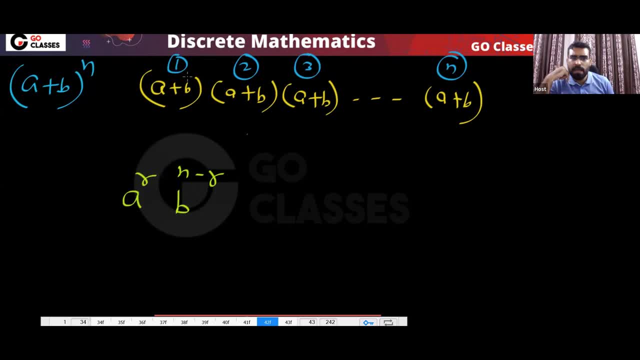 automatically, number of b will be from the remaining b will come. If from here, if from r places a is coming, then from remaining places total n places you have. If from n r places a is coming from remaining places, b will come. Okay, So in how many ways you? 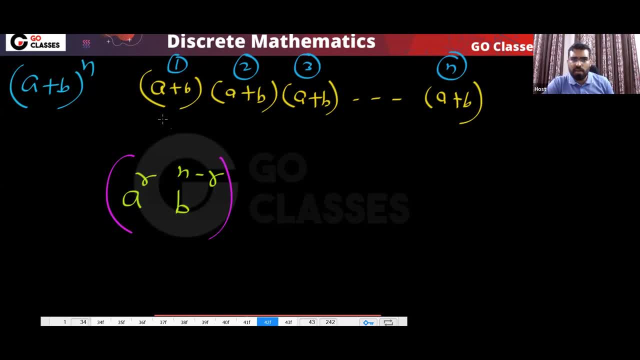 can get this, How many ways You can decide from these n you can decide who will give you a. From these n you can decide, you can decide r of them who will give you a. So this is the idea. And finally, 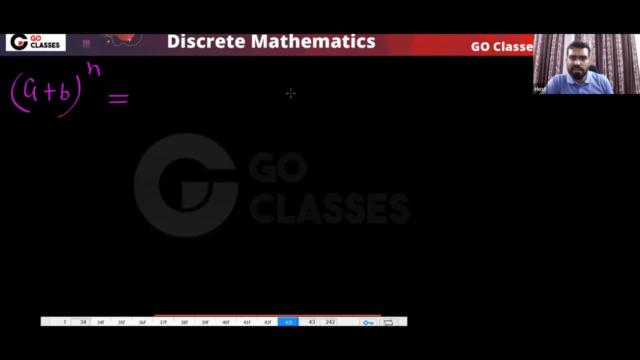 if I want to say that a plus b power n, then how can I say? I can say that. I can say every term will have a power r, b power n minus r. Every term will be like this, And how many such terms we have. 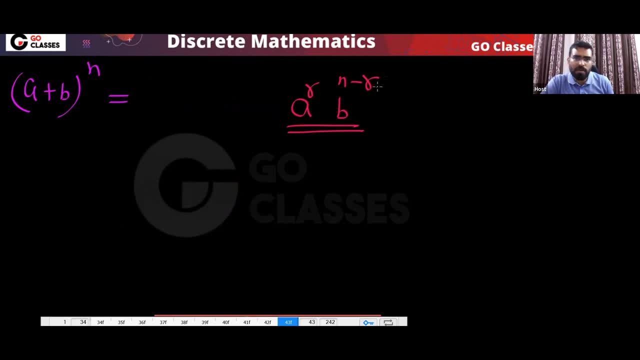 Every term will be like this: If you have a power, r, then b power will be n minus r. How many such terms you can create From n. you can decide who will give you which r will give you a. And this r can go from where to where This power can go from where to. 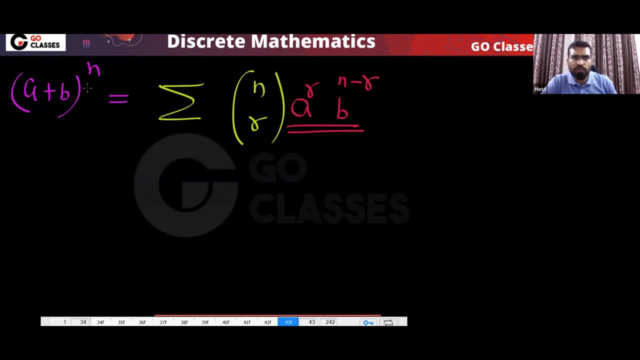 where This power, number of a number of a can go. number of a can go from 0 to n. Okay, This is your answer. You know nкр is equal to ncn minus r. You know that ncr is equal to n minus r, So you, 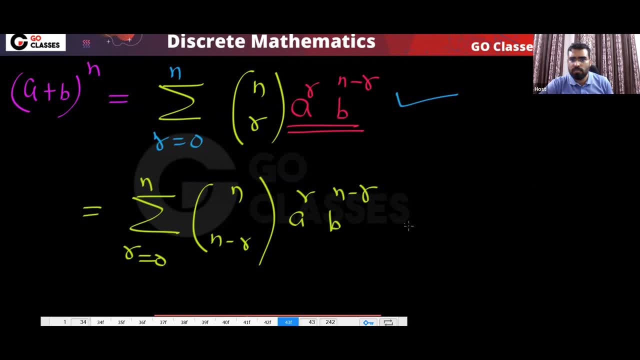 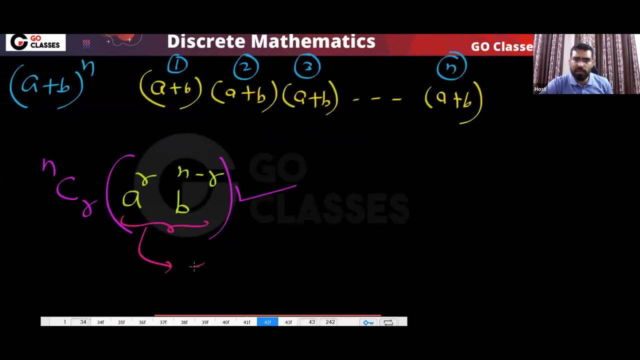 can write like this, also, like this also. you can write: Okay, This is your binomial theorem, This is the binomial theorem. Did you understand the proof of binomial theorem? Basically, every term will be like this, Every term will be like this, Every term, every. 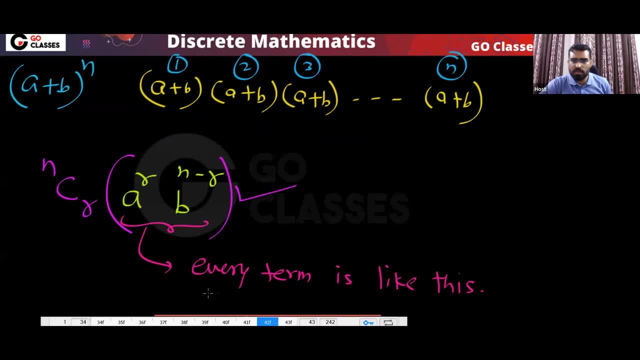 term is like this is like this: okay, if you have r a, then you will have n minus r b. okay, if your number of a's are- if you are taking number of a's are- then how many b's will be there if you are taking r a's? 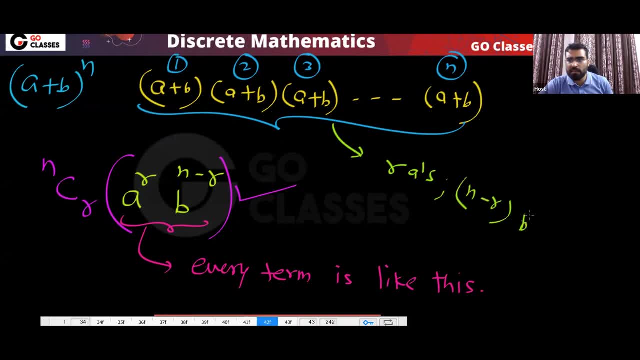 then automatically, automatically, n minus r b's will be there, then automatically n minus b is okay now. so every term will be like this. and in how many ways i can create this term ncr. these many ways i can create this term i can decide from these n. there are total n. 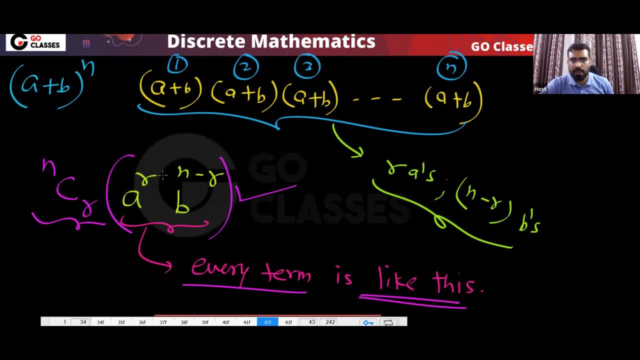 from these n i can decide who will give me a, which r of them will give me a. so, from these, and i can select r of them, they will give me a ncr. they will give me a. they will give me. is okay, these are people they will give you, is so? finally, i can say that this number of a 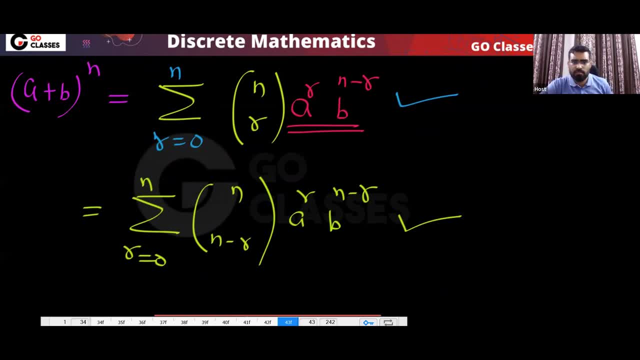 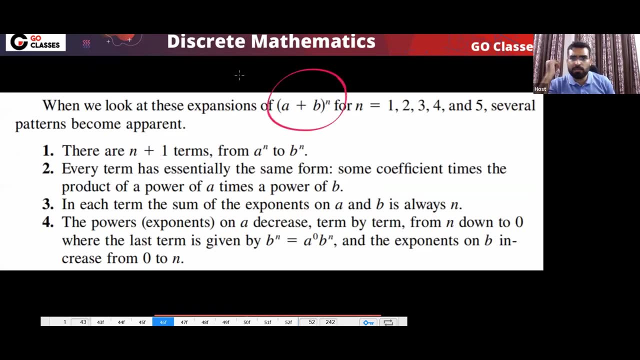 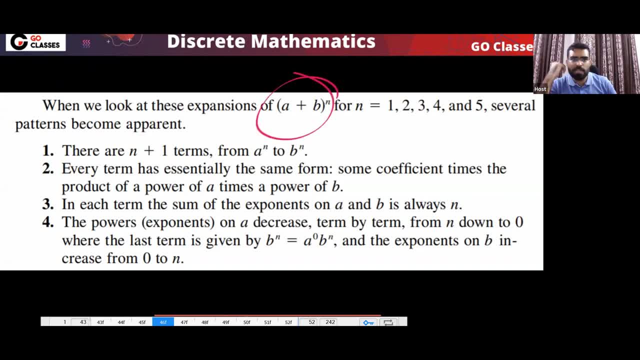 they can ask you how many terms will be there in this expansion: a plus b power n. how many terms will be there in the expansion? n plus one terms will be there. why there will be n plus one terms. for example, what is a plus b power four? 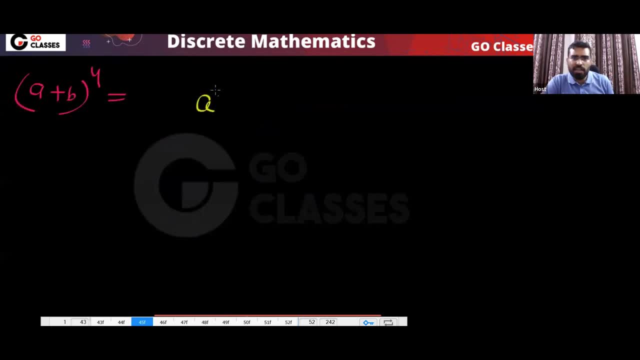 why there will be n plus one terms. for example, what is a plus b power four? a plus b power four is like this: you can have a power a plus b power. four is like this: you can have a power a plus b power four is like this: you can have a power zero. then how many b will be there? 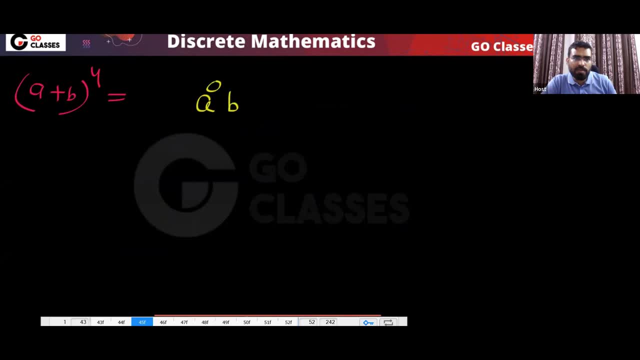 zero, then how many b will be there? zero, then how many b will be there? if you have a power zero, then how many b. if you have a power zero, then how many b. if you have a power zero, then how many b will be there, for example, maybe 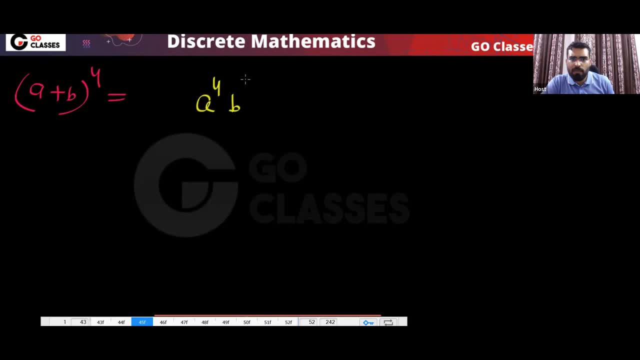 will be there. for example, maybe will be there. for example, maybe. if you have a power four, then how many b. if you have a power four, then how many b. if you have a power four, then how many b will be? there will be. there, will be there. if you have a power four, then number of b. 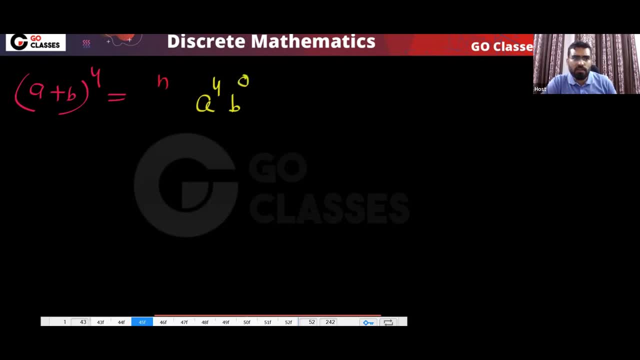 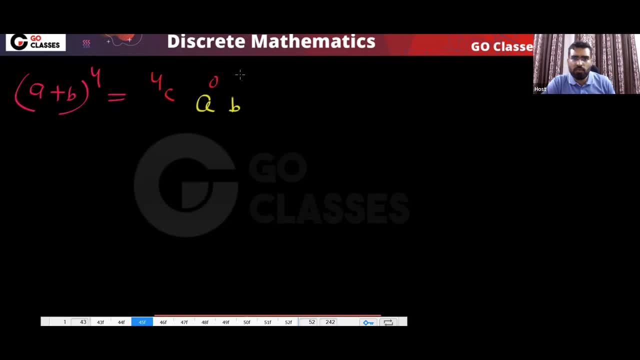 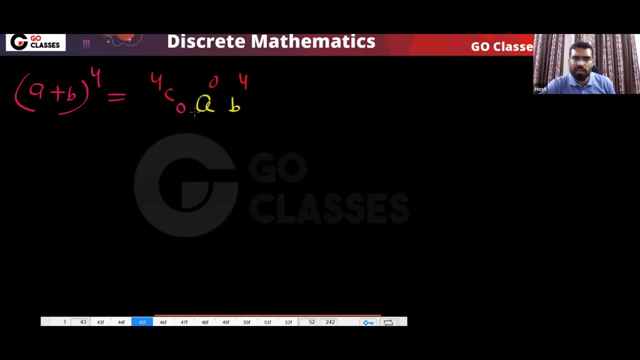 anyway, all are all are same, okay. so if you have a power zero, then you have a power zero, then you have a power zero, then b power will be four, so you can decide. b power will be four, so you can decide. b power will be four, so you can decide who will give you. 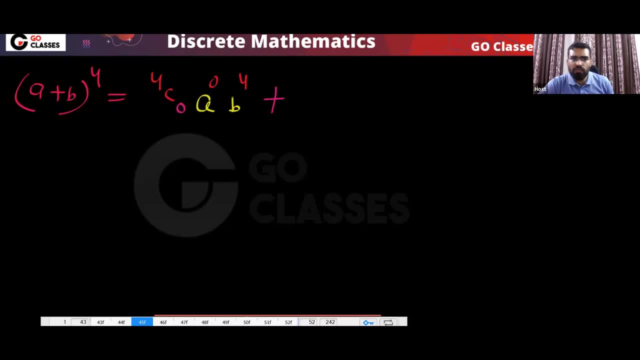 who will give you who will give you a. none of them will give you a. you can a. none of them will give you a. you can a. none of them will give you a. you can decide who will give you one a here you decide who will give you one a here you. 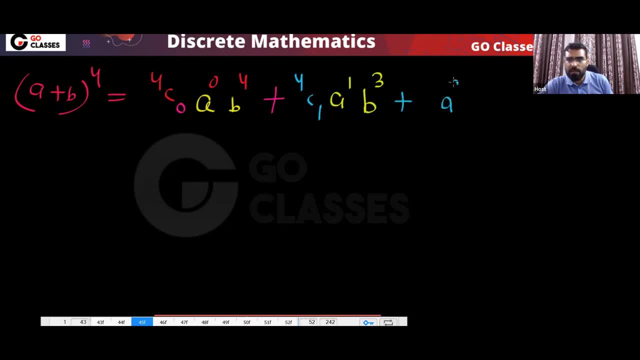 decide who will give you one a. here you can decide who will give you zero a. can decide who will give you zero a. can decide who will give you zero a. if a power two, then b power automatically. if a power two, then b power automatically. if a power two, then b power automatically will be two. 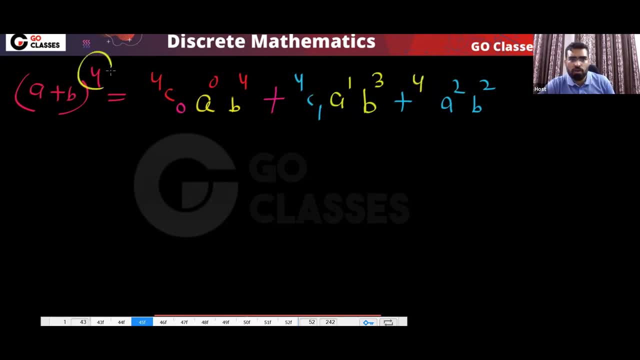 will be. two will be two. you can decide who will give you two a's. you can decide who will give you two a's. you can decide who will give you two a's from these four. from these four, who will? from these four? from these four, who will? 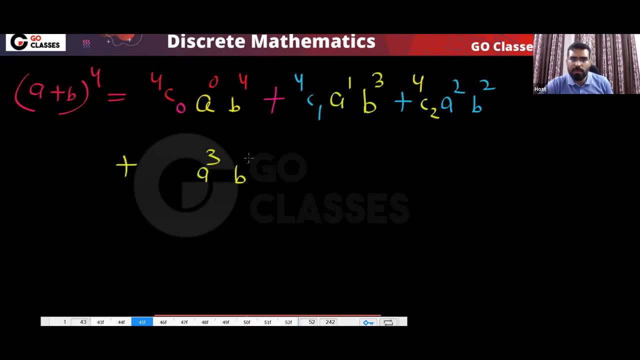 from these four? from these four, who will give you two a's? give you two a's. give you two a's plus. if a power three, then b power will give you two a's plus. if a power three, then b power will give you two a's plus. if a power three, then b power will be one. you can decide who will give you. 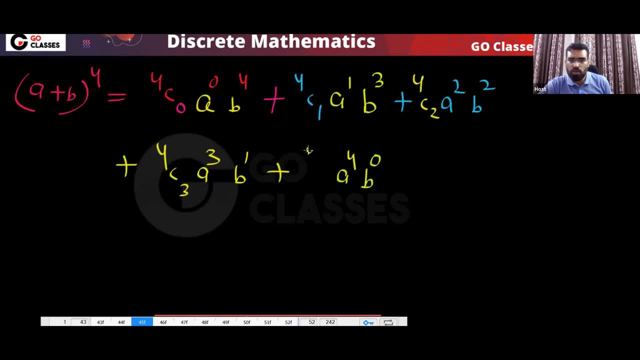 be one, you can decide who will give you. be one, you can decide who will give you three a's, three a's, three a's. if a power four, then b power zero you can. if a power four, then b power zero you can. if a power four, then b power zero. you can decide who will give you four a's. 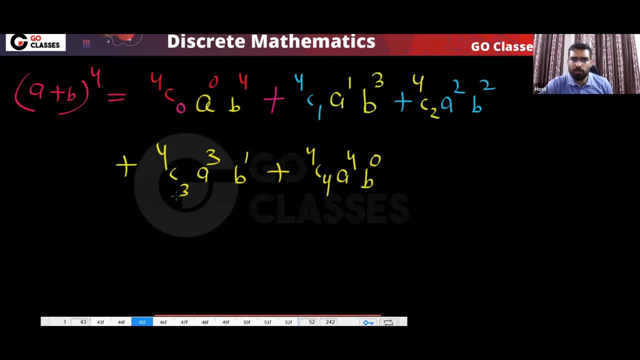 decide who will give you four a's. decide who will give you four a's. that's it. no other term is possible. only that's it. no other term is possible. only that's it. no other term is possible. only these are possible, these are possible, these are possible. so you cannot. this is nothing but. 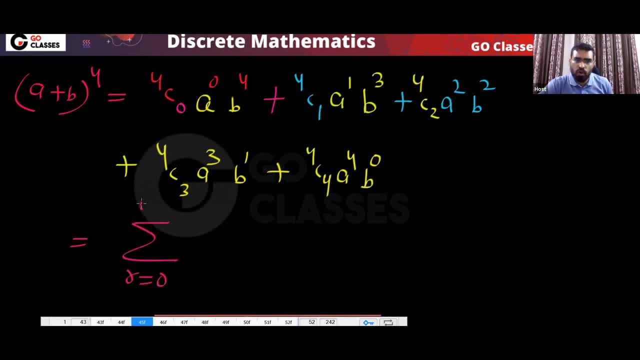 so you cannot. this is nothing, but so you cannot. this is nothing but summation, summation, summation: r is going from zero to four. r is going from zero to four. r is going from zero to four. you have ncr. you have four c. you have ncr. you have four c. 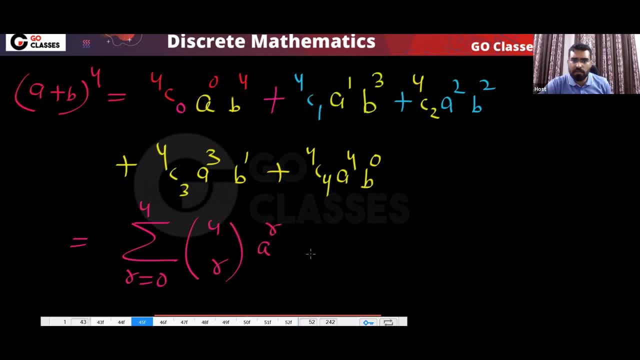 you have ncr, you have four c, four cr. and if you have a power r, four cr, and if you have a power r, four cr, and if you have a power r, then you have b power four minus r, then you have b power four minus r. 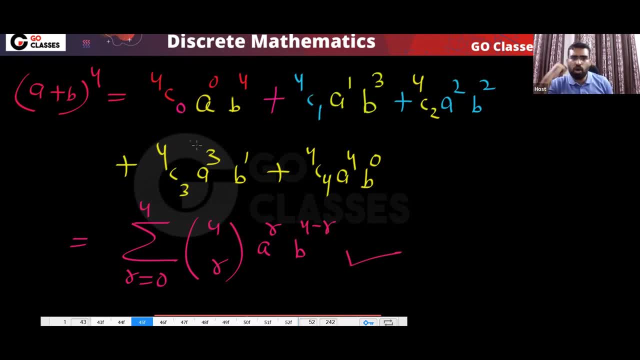 then you have b power four minus r. this is the expression. this is the expression. this is the expression. is it clear to everyone? so, how many is it clear to everyone? so, how many is it clear to everyone? so, how many terms we have in this, a terms we have in this: a. 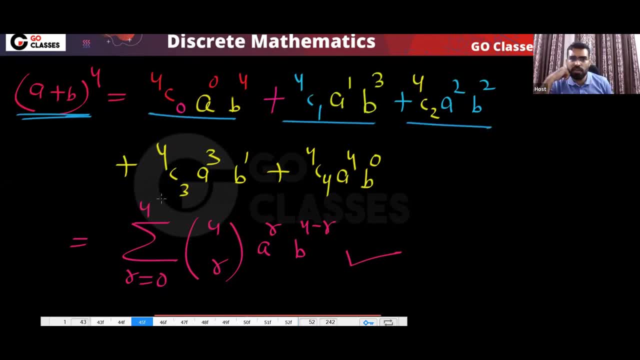 terms: we have in this: a in this a plus b, power four. in this: we in this: a plus b, power four in this we in this a plus b, power four. in this we have one, have one, have one, two, three, four, five, so total five terms. two, three, four, five, so total five terms. 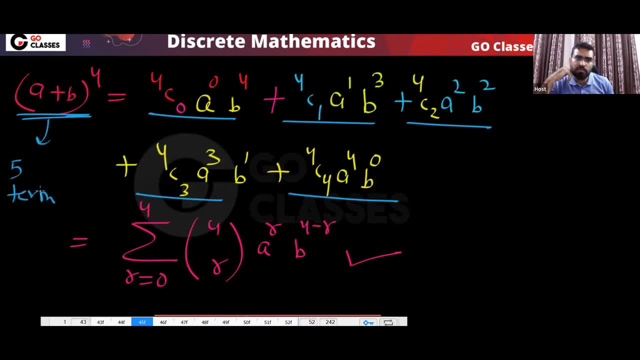 two, three, four, five, so total five terms. we have, we have, we have, so this will have total five terms. so this will have total five terms, so this will have total five terms. okay, so similarly, this n plus once this. okay, so similarly, this n plus once this. 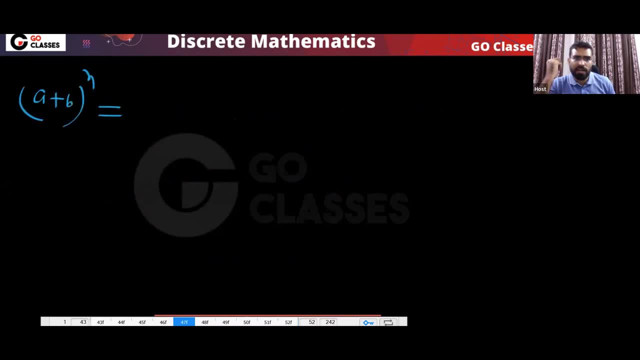 okay, so similarly, this n plus once this: uh this a plus b power n uh this a plus b power n uh this a plus b power n this a plus b power n. this will have how this a plus b power n. this will have how this a plus b power n. this will have how many terms total, because the formula 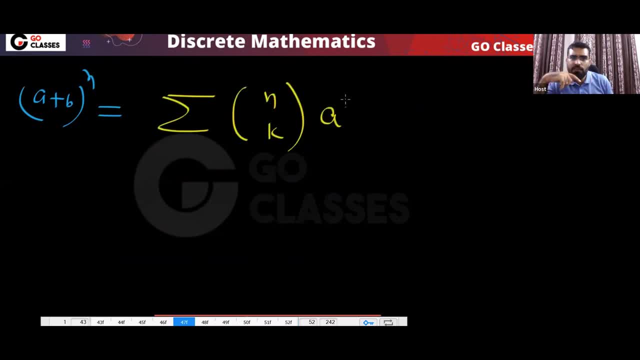 many terms total because the formula. many terms total because the formula is like this, is like this, is like this. the formula is like this: n c k. if you the formula is like this: n c k. if you the formula is like this: n c k. if you have k a's, then number of b's will be: 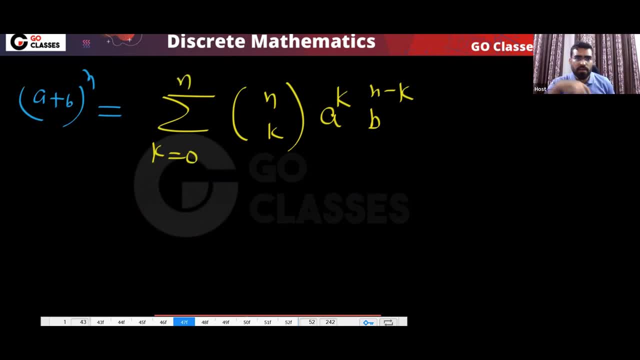 have k a's, then number of b's will be: have k a's, then number of b's will be n minus k, and this k is going from zero: n minus k. and this k is going from zero: n minus k. and this k is going from zero to n. 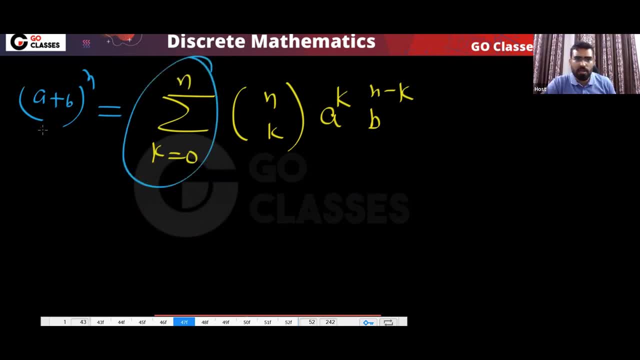 to n to n. so because this k is going from zero to so, because this k is going from zero to so, because this k is going from zero to n, so how many terms? n so how many terms? n so how many terms? because this k is going from zero to n, so 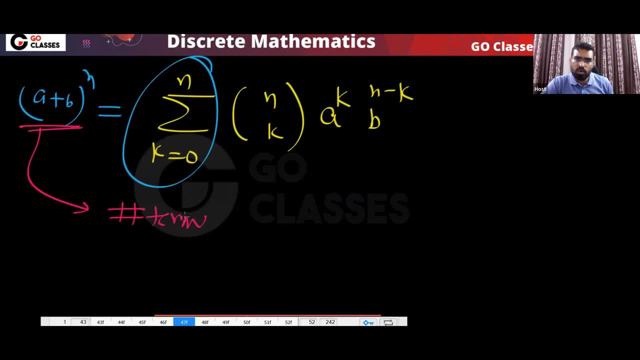 because this k is going from zero to n. so because this k is going from zero to n, so how many terms, how many terms, how many terms. so number of terms will be. because this so number of terms will be, because this so number of terms will be, because this k is going from zero to n, so number of 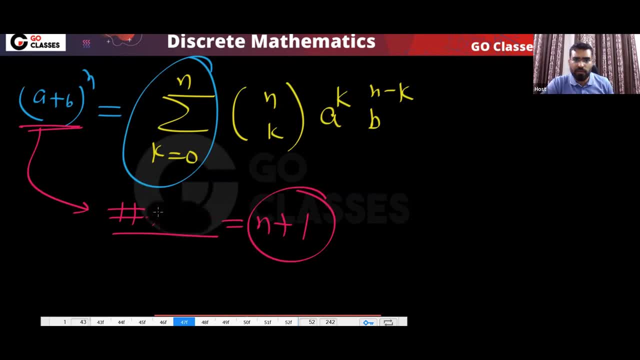 k is going from zero to n, so number of k is going from zero to n, so number of terms will be n plus one. terms will be n plus one. terms will be n plus one. so these many terms you will have, so these many terms you will have. 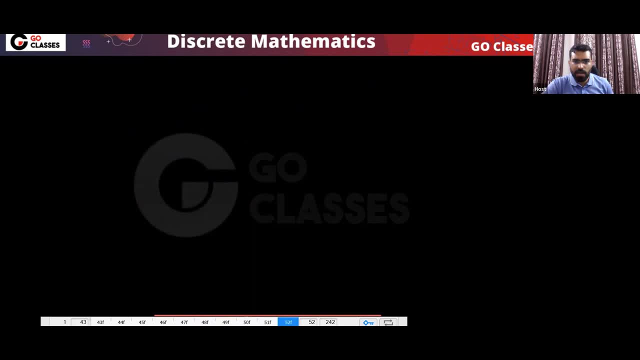 so these many terms you will have, okay, let's move on, okay, let's move on, okay, let's move on. so this is the binomial theorem, and so this is the binomial theorem, and so this is the binomial theorem. and these are the statement. these are the statement. 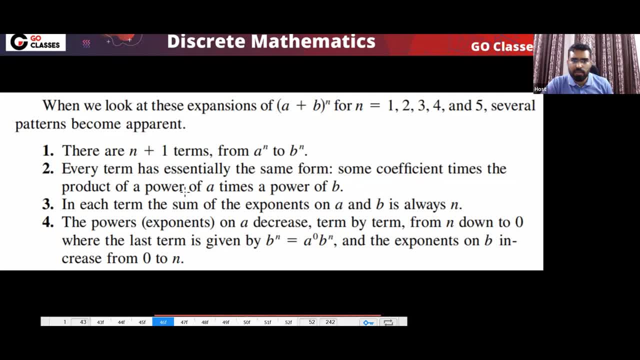 these are the statement. so, first of all, there will be n plus one. so, first of all, there will be n plus one. so, first of all, there will be n plus one terms in every term terms, in every term terms, in every term. you will have, okay, uh, every term you. 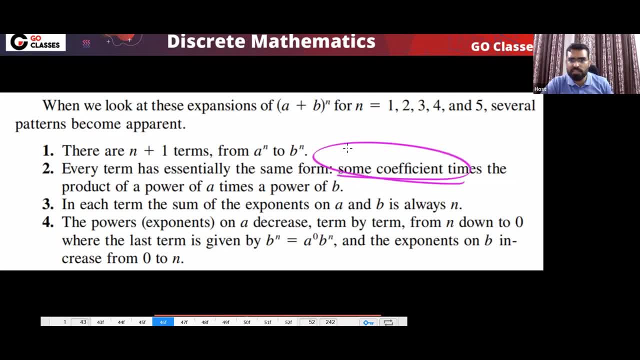 you will have, okay, uh, every term you. you will have, okay, uh, every term you. power of b and number of summation of power of b. and number of summation of power of b. and number of summation of exponent. summation of power of a comma. 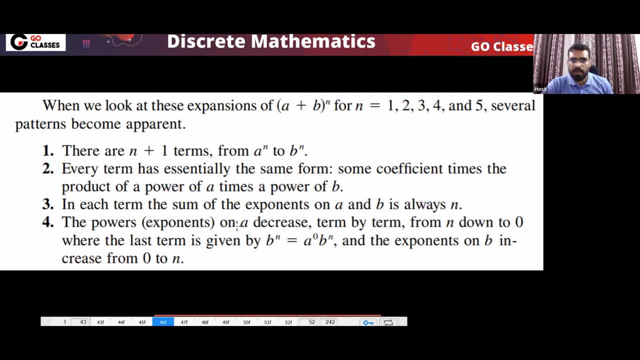 exponent summation of power of a comma. exponent summation of power of a comma: b. that will always be b, that will always be b, that will always be n, and if a power is increasing, then b? n, and if a power is increasing, then b n, and if a power is increasing, then b power will decrease. 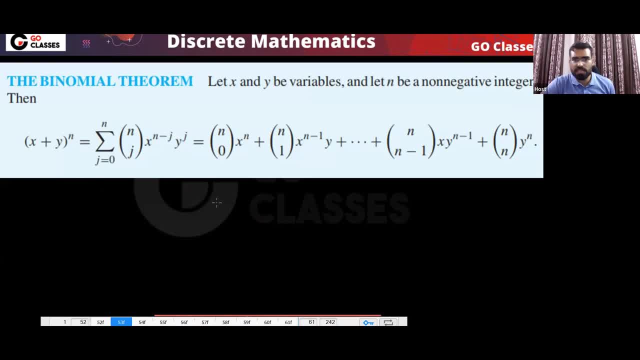 so this is your binomial theorem, isn't so? this is your binomial theorem, isn't so? this is your binomial theorem, isn't it simple, it simple, it simple. this is the binomial theorem x plus y. this is the binomial theorem x plus y. 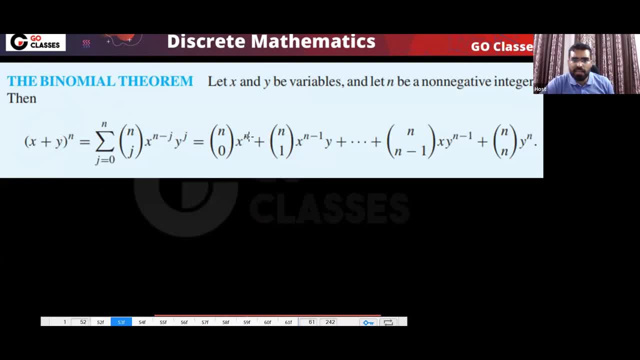 this is the binomial theorem: x plus y power n, that will be power n, that will be power n, that will be just decide. if you are taking for, just decide, if you are taking for, just decide, if you are taking, for example, if you are taking x power n, then 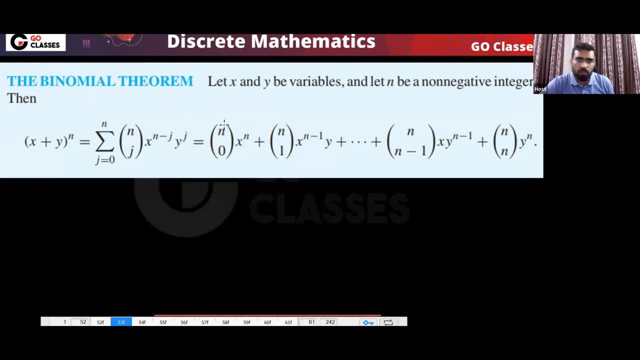 example, if you are taking x power n, then example: if you are taking x power n, then y power 0, y power 0, y power 0. so just decide who will give you power 0. so just decide who will give you power 0. so just decide who will give you power 0. who will give you uh y power 0, so nc0. 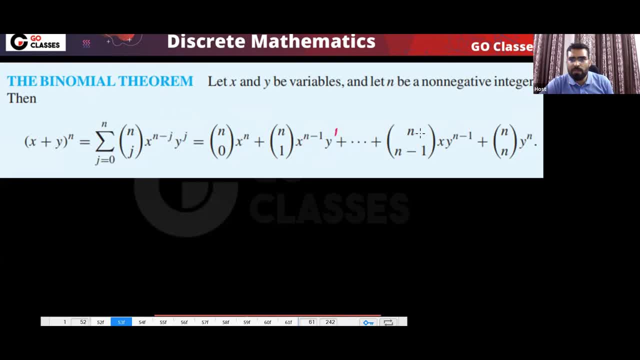 who will give you uh y power 0 so nc0. who will give you uh y power 0 so nc0. who will give you y power 1 so nc1. who will give you y power 1 so nc1. who will give you y power 1 so nc1. who will give you y power 2 nc2. 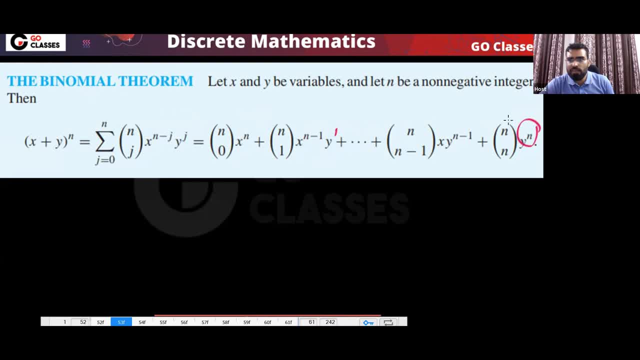 who will give you y power 2 nc2. who will give you y power 2 nc2? here we. who will give you y power n minus here we. who will give you y power n minus here we. who will give you y power n minus one ncn minus one. who will give you y. 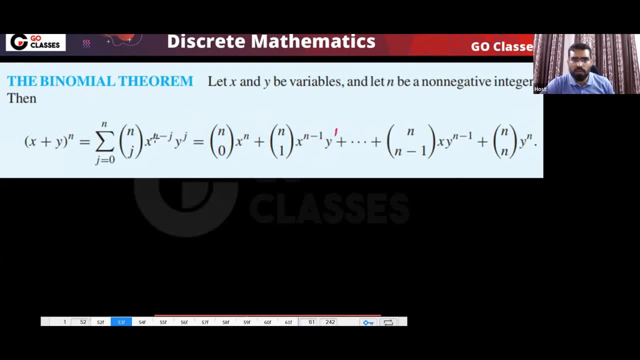 one ncn minus one who will give you y. one ncn minus one who will give you y power, n power, n power n ncn. so if x power is n minus j ncn, so if x power is n minus j ncn, so if x power is n minus j, then y power will be j and this j. 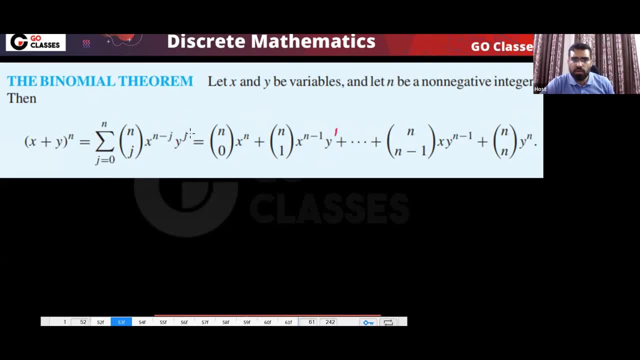 then y power will be j and this j, then y power will be j and this j? y power. this can go from 0 to n? y power. this can go from 0 to n? y power. this can go from 0 to n, and you can decide who will give you y. 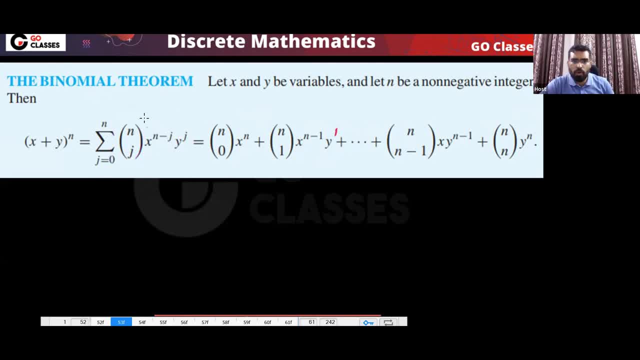 and you can decide who will give you y. and you can decide who will give you y power, j power, j power, j. so from n. j will give you from n. you can. so from n. j will give you from n. you can so from n. j will give you from n. you can select j. 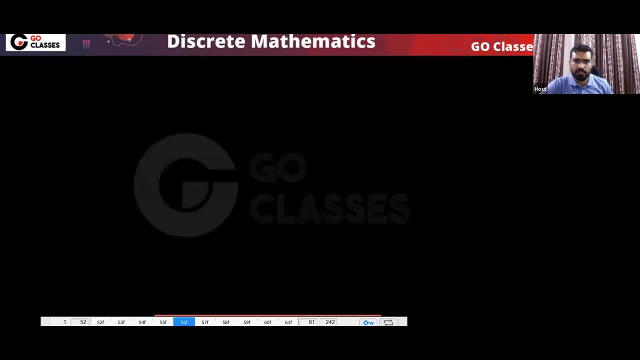 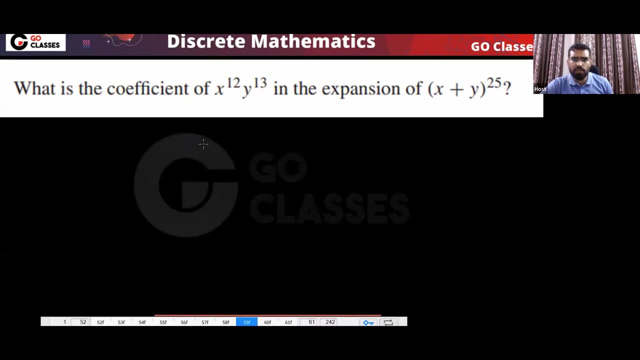 select j. select j. those will give you y. this is your x plus y power 4. tell me this is your x plus y power 4. tell me this is your x plus y power 4. tell me the answer for this. what is the coefficient of x power 12 y? 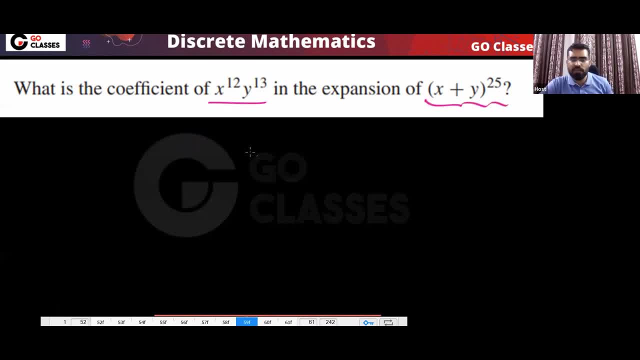 what is the coefficient of x power 12- y? what is the coefficient of x- power 12, y power 12- power 12 in the expansion of x plus y power 12 in the expansion of x plus y power 12 in the expansion of x plus y power 25. 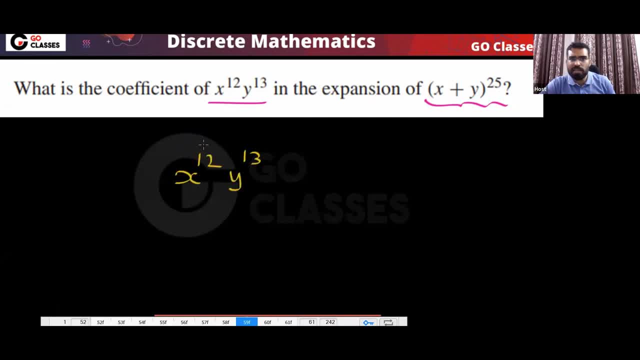 power 25, power 25. so x, power 12, y, power 13. first you tell so x. power 12, y, power 13. first you tell so x power 12, y, power 13. first you tell me: is this possible, me, is this possible, me, is this possible? x power 12, y, power 13: is this possible? 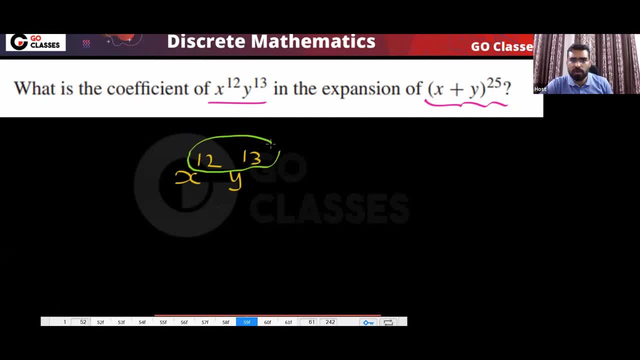 yes, this is possible. right because this- yes, this is possible. right because this- yes, this is possible, right because this is possible- is possible because 12 plus 13, that is equal to 25, is possible because 12 plus 13, that is equal to 25. 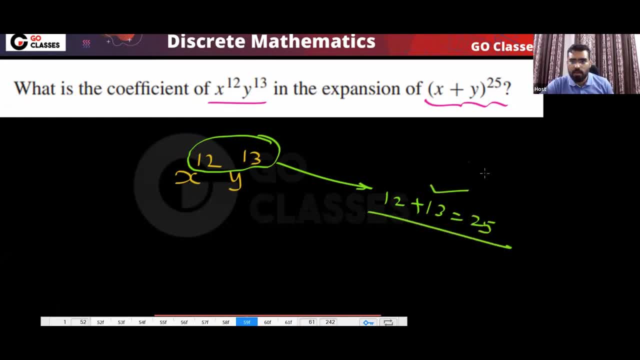 is possible, because 12 plus 13, that is equal to 25. so this is definitely possible. so this is definitely possible. so this is definitely possible. and next, okay, so how many terms? so, and next okay, so how many terms? so, and next okay, so how many terms? so, total 25 terms you have. 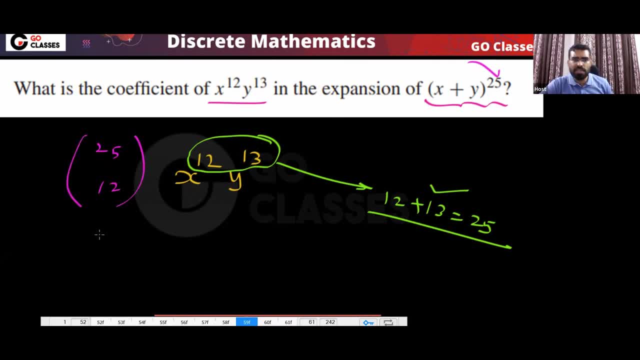 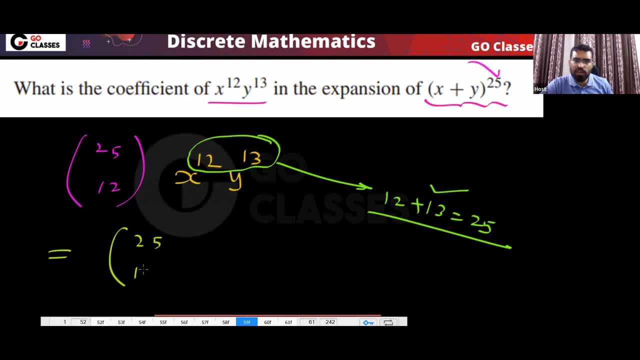 you can decide who will give you x, and this is same as you can also decide- and this is same as you can also decide- you can also decide who will give you y. you can also decide who will give you y. so the answer will be. answer will be: you can decide who will give you x, and that is same as you can also decide. 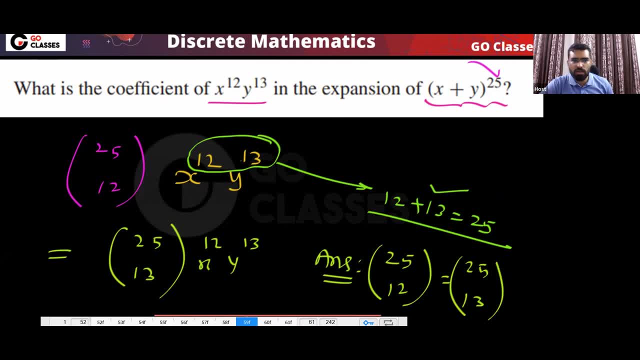 who will give you y? both are same, so your answer will be 25, c12. if i ask you now, tell me what is the answer: x power 12, y power 14. so what is the coefficient of this? so the coefficient of this, that will be 0, 0 will be the coefficient of this. so here, what is the answer? answer will be 0. 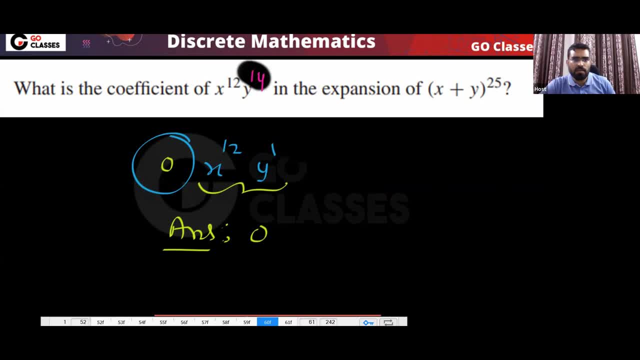 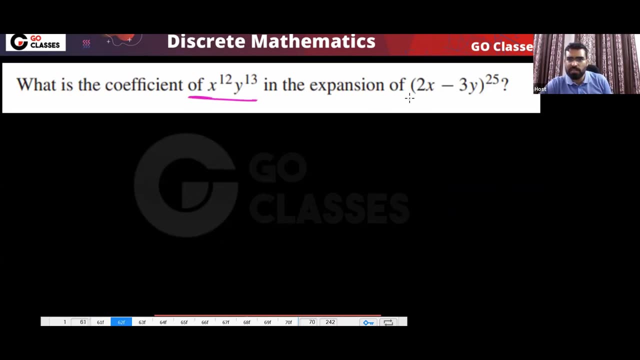 because this is never possible. see, this is never possible because, if you notice, then this, 12 plus 14, this is not equal to 25.. okay, tell me the answer for this. what is the coefficient of x power 12 by power 13 in the expansion of this? 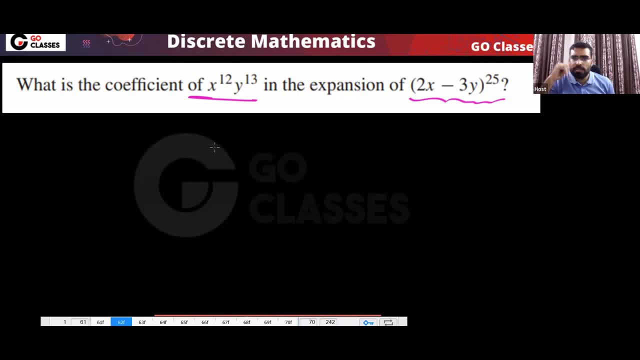 i won't first. is it possible? is this possible? yes, of course it is possible. you can check. it will be possible. now, what is the answer? so you can think like this: you can think a as 2x and you can think b as minus 3y. this is how you. 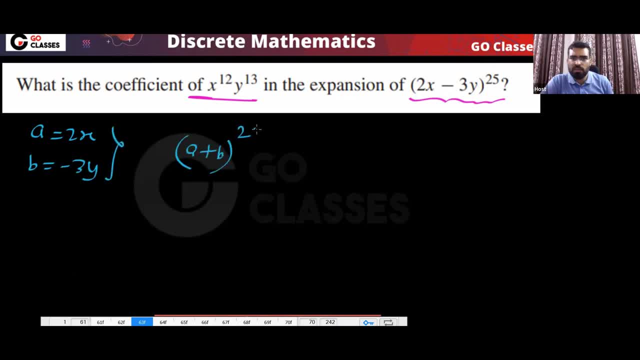 can think. so you have a plus b plus power 25. this is what you have. this is what you have. okay, so in this, basically, what we want, we want a power, we want a power 12, we want b power 13.. this is what we want. so that will be 25 c12. now. what is your a now? what is your a? 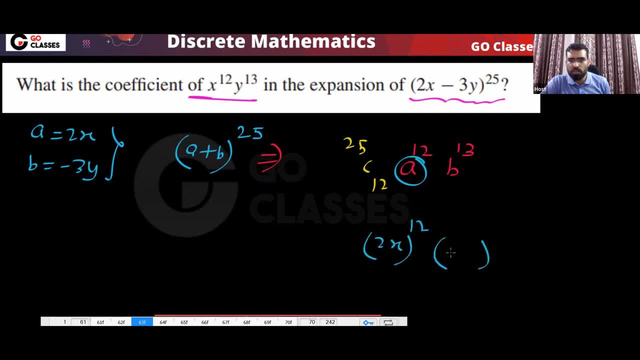 a is basically 2x, 2x power 12.. what is your b? b is minus 3 y, power 13.. 25, c12. the question is asking: what is the coefficient of x power 12, y power 13.. so x power 12, y power 13, the coefficient will be: 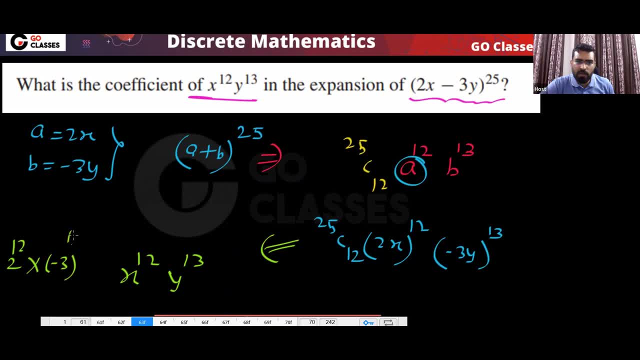 2 power 12 multiplied by minus 3 power 13 multiplied by 25: c12. this will be the answer. okay, because we are only interested in this. this is what we want. we only want x power 12, y power 13.. so the answer will be: so, finally, what is the final answer? 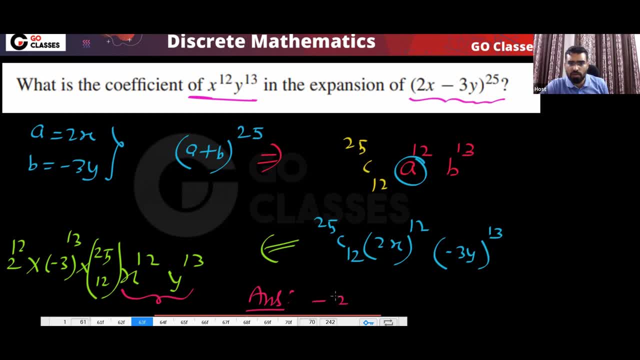 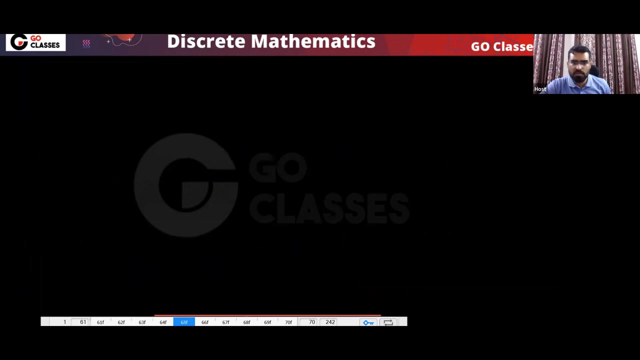 tell me the final answer. final answer will be minus of minus of 2 power 12, 3 power 13, multiplied by 25: c12. this will be your answer. okay, is this clear? because we want, we want this, this is what we want, so the coefficient will be this. next question, next question. so 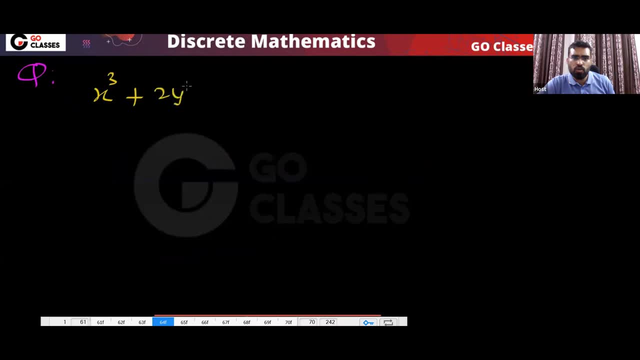 let's assume you have x power 3 plus 2 y power, 2 power 10. okay, then my question is: what is the coefficient of, what is the coefficient of? i can ask you, what is the coefficient of x power? so, basically, this type of question they can ask you. 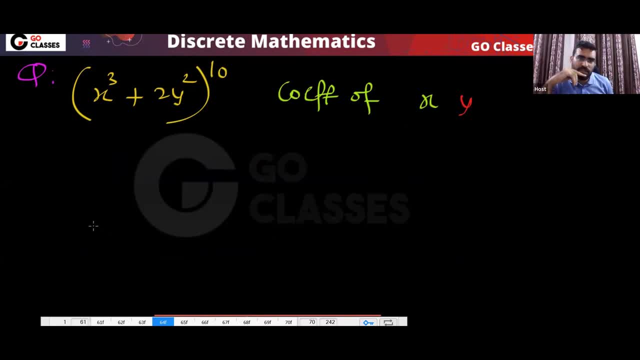 okay, x power 3. so every term that you will create here, every term that you will get, that will be like: so this x power 3 power, something will be there, and 2 y square power 10 minus r will be there. so what i can do, i can do. maybe, if i take, so i can do 12 okay. so tell me the answer for this. 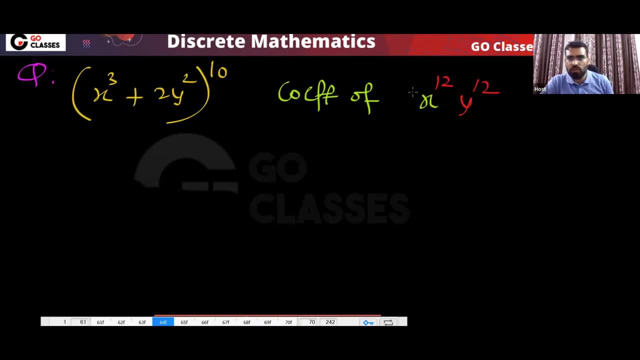 tell me the answer for this. what is the coefficient of, what is the coefficient of this? i am asking coefficient of this, so tell me the answer. i am asking coefficient of this. coefficient of 2x power 12, y power 12.. What will be the answer? So you can notice that, first of all, 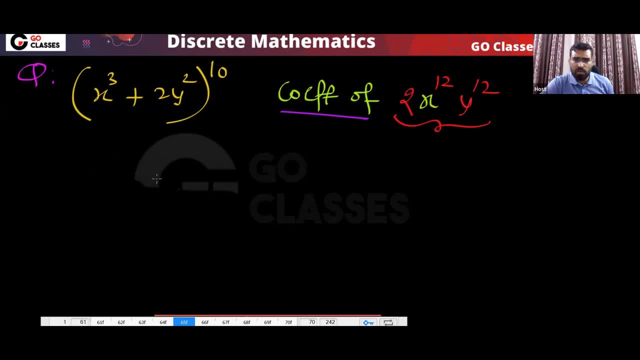 you want x power 12. You want x power 12. So what do you need? If you want x power 12, then you need its power 4. Its power 4, you want. Its power 4 you want, Then automatically. 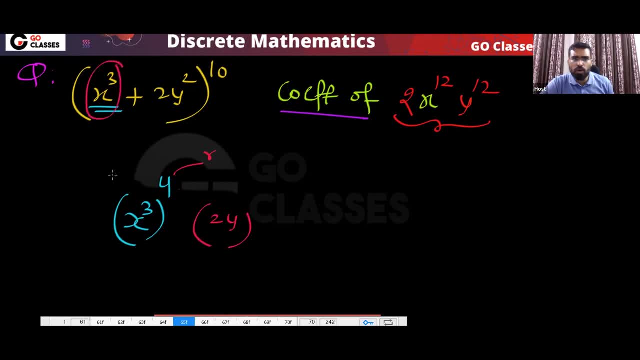 what will be the? if you want power 4, for this you want power 4.. Then automatically, this will have what power, This will have what power. So, 2y square, This 2y square, this power will be 10 minus 4.. Okay, Yes or no, Its power will be 10 minus 4.. And how? 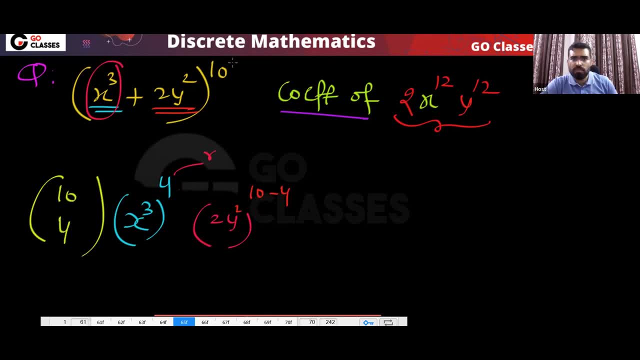 many times you can create this, that will be 10c4.. That will be 10c4.. Because this is your r, So I can say 10c4 times you can create this. So from here what we got, We got x power. 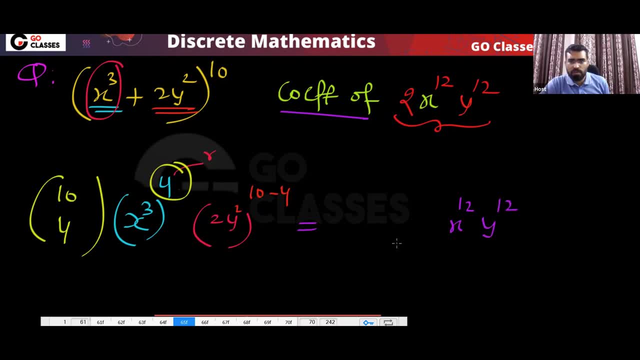 12, y power 12.. What else we got? We got 10c4.. What else we got? We got 2 power 6.. So I can write like this: Now the question is asking: what is the coefficient of this? So the answer: 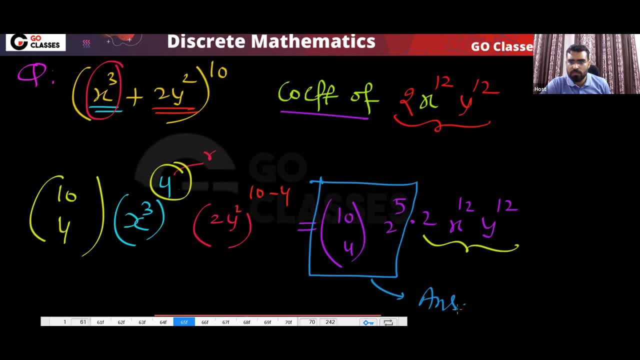 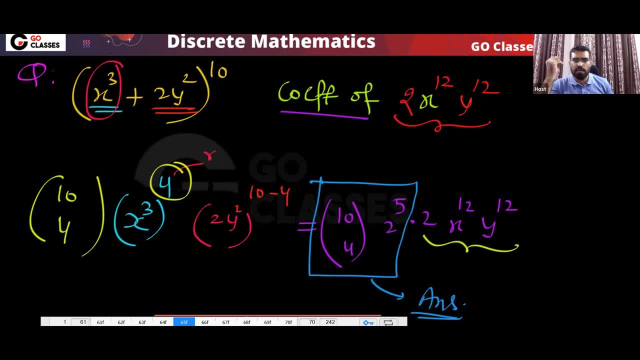 The answer will be 10c4, 2, power 5.. Is it clear? Is this clear to everyone In the same question? if I do, in the same question, let me change. If I do, y, power 14.. Now, what will be the answer? 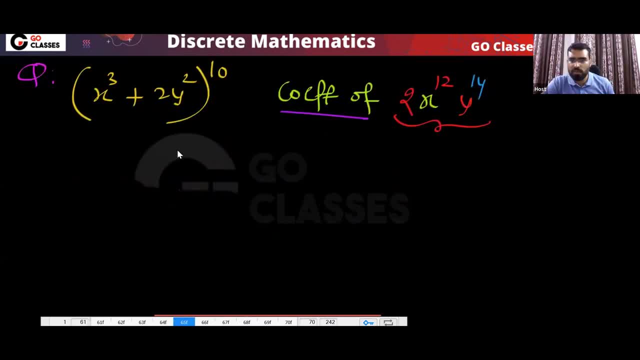 In the same question. If I do y power 14.. Now the coefficient will be: What will be the coefficient Here? the answer will be 0.. The coefficient will be zero, Because see, what do you want? You want x, power 12.. 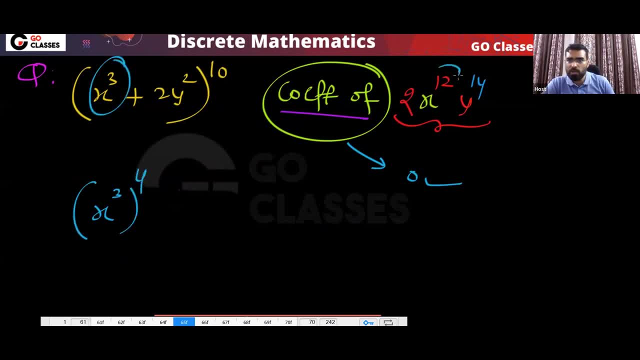 So this term you want 4 times, Because you want x, power 12, this is what you want. This is what you want. So this term you want total 4 times This you want. Then automatically, automatically, this will come 6 times. 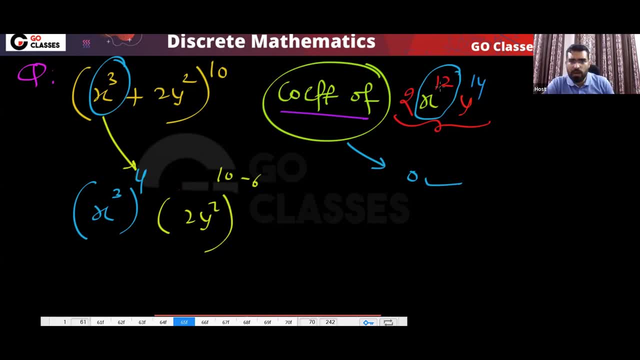 Then automatically this will come 6 times. So you can notice: if you have x power 12, then automatically y power will be 12.. Y power will not be 14.. So here the answer will be zero. Okay, So for this answer will. 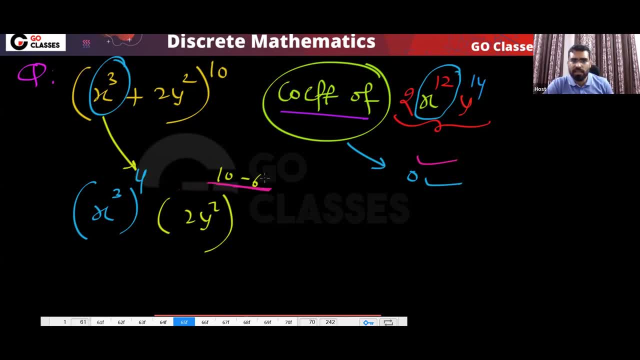 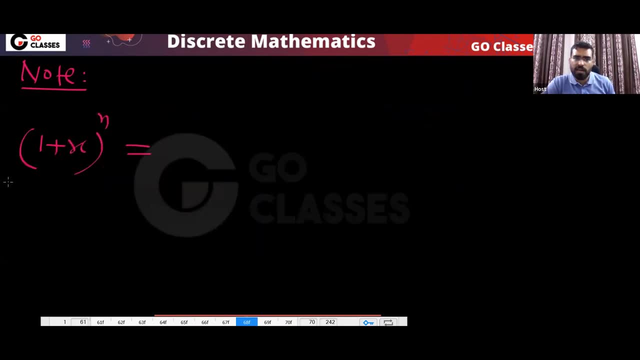 be zero. So this is the idea. So you can get only Y power 12.. Like this you can handle all these things. What is one plus X power? N? Like if one of them has fixed, then what? that will be? NC0 X power zero. NC1 X power one, NC2 X power two, and so on. NCN X power. 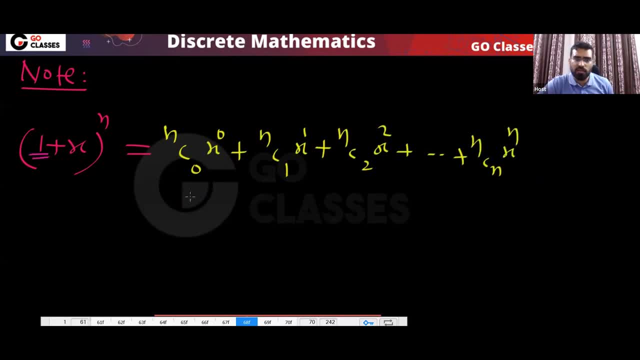 N. Right, Because this is already one. This is fixed. This is one, So I can say: like how many X will be there? So you can think like this: So if X is zero, then you can decide who will give you zero X, So NC0.. If X is one, then NC1.. If X is two, then NC2.. If X is. 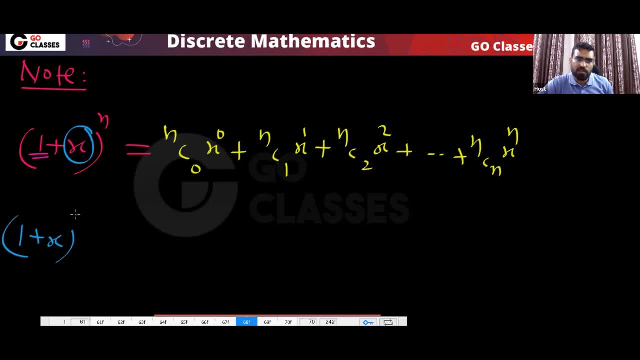 power N. then. So what is this? Finally, what is this? This is basically X power. This will be one plus. Okay, It will be like this: You will have one plus X power N. NC1 X plus NC2 X square, NC2 X square plus NC3 X cube, and so on. NCN X power N. So this: 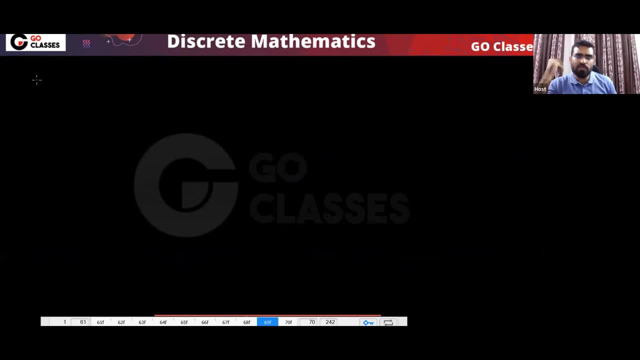 will be your formula. Now if I put: if I put X equal to one in this, if I put X equal to one, what will happen? Put X equal to one, What will happen? Put X equal to one? Put X equal to one, then what? Let us say, this is the adaptive action. 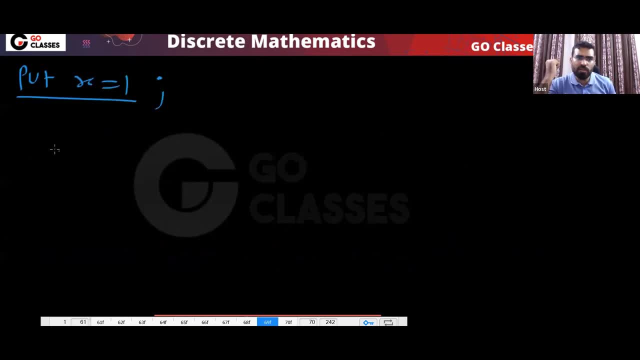 So put X equal to one. If you put X equal to then one, what will happen? You will get two power N. This will become two power N And this will become NC0 plus NC1 plus NC2 and CN. And this is your summation of binomial coefficients, Yes or no? This is your summation. 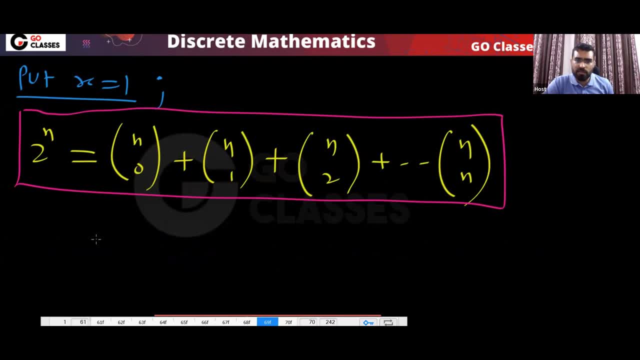 of binomial coefficient. We have already seen this. This is another way. The same thing you can do in many different ways. So this is your ncr summation: ncr where r is going from 0 to n. So this will be 2 power n. Just put x equal to 1.. If you put x equal to 1, 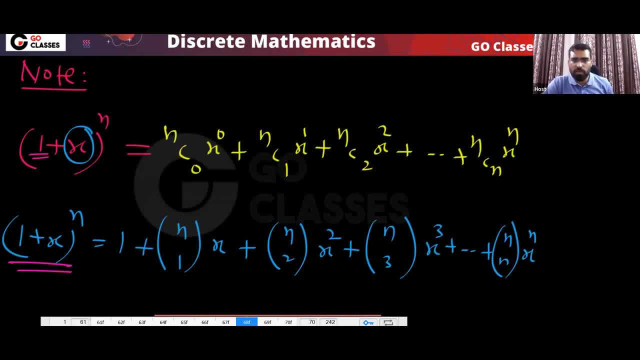 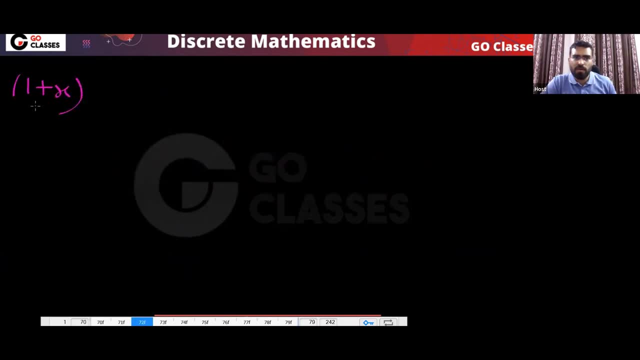 this will become 2 power n. And if you put x equal to 1, then this will become summation of binomial coefficients: Put x equal to 1.. So remember, in 1 plus x power n- this you already know, this is your nc0 plus nc1 x plus nc2 x square, and so on: ncn x power n. Put x equal. 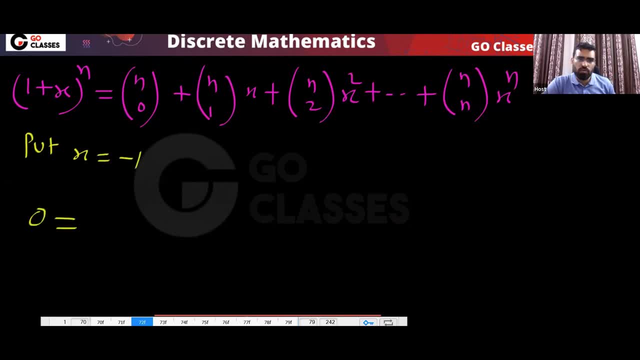 to minus 1.. Then you will get 0.. 0 equal to 0 equal to, because you are putting x equal to minus 1.. So this will be like this: nc2 minus, nc3 plus. Alternative plus minus will go on.